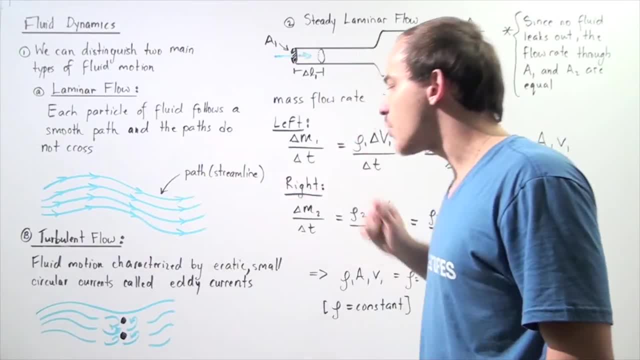 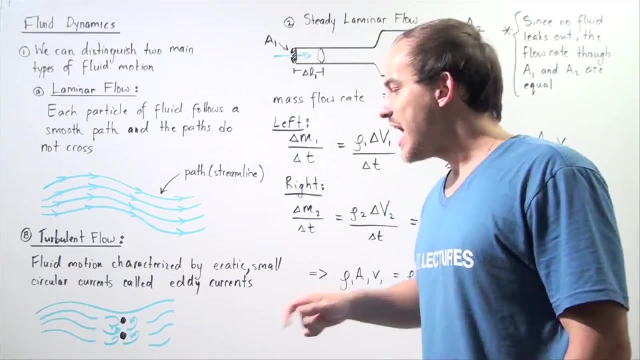 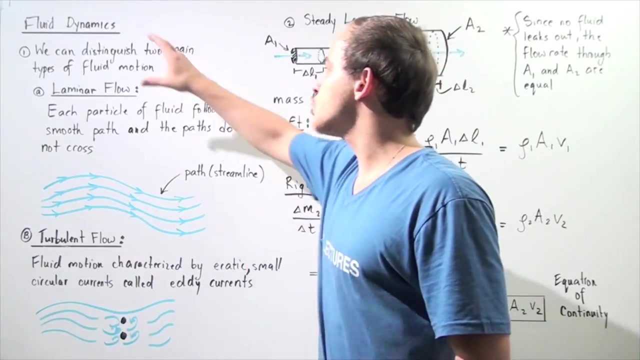 and that's because turbulent flow is characterized by erratic, small circular currents called eddy currents, also known as eddies, as shown in the following diagram. So these eddies create a lot more resistance than compared to laminar flow, where there is less resistance. 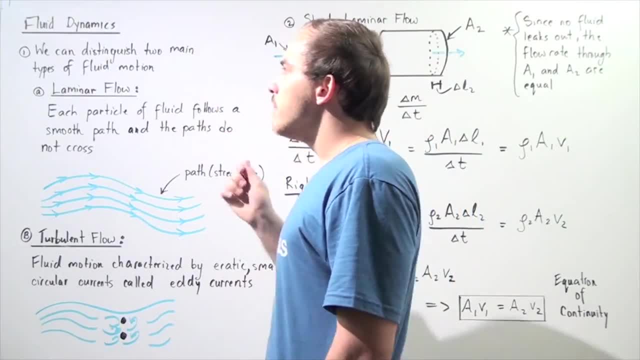 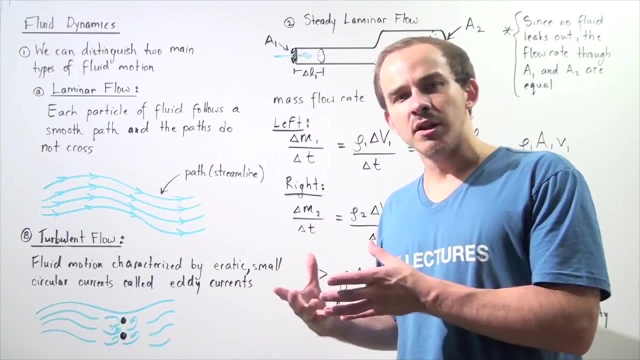 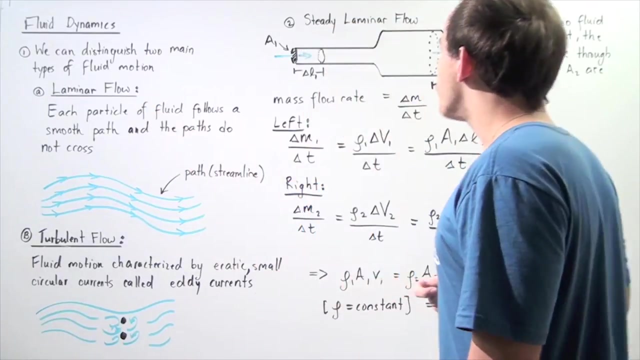 Now let's examine laminar flow much more closely. Let's try to come up with an equation that will help us deal with problems in which fluids are experiencing laminar or streamlined flow. So let's suppose that we have the following pipe: 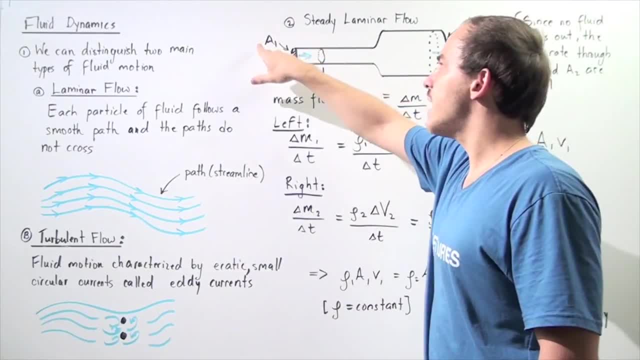 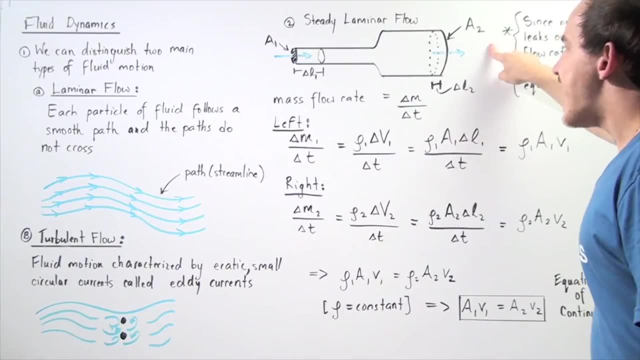 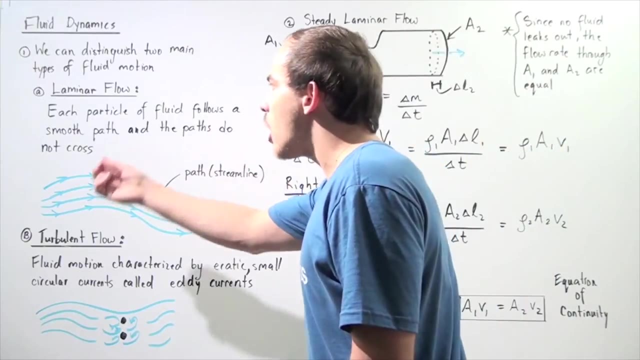 on the left end of the pipe we have cross-sectional area A1, and on the right side of the pipe we have cross-sectional area A2.. Now let's assume that inside the pipe we have a certain fluid that is flowing via laminar flow. 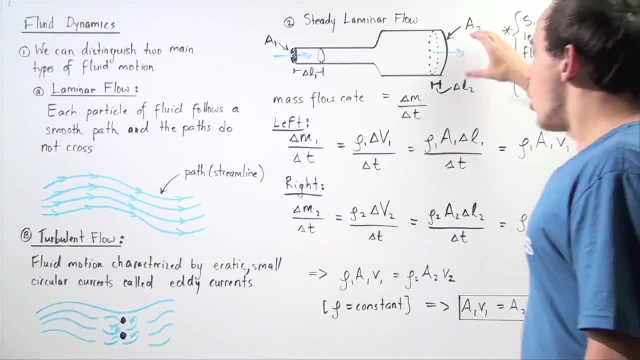 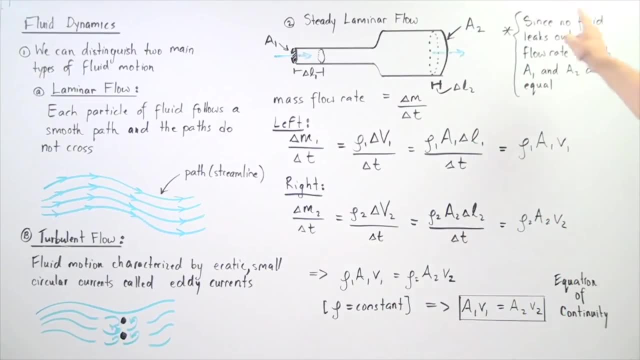 so steady, streamlined flow. Let's also assume that there are no leaks or holes within the pipe and that means, since no fluid leaks out, the flow rate through area A1 and area A2 are exactly the same. So whatever amount of fluid that comes in, 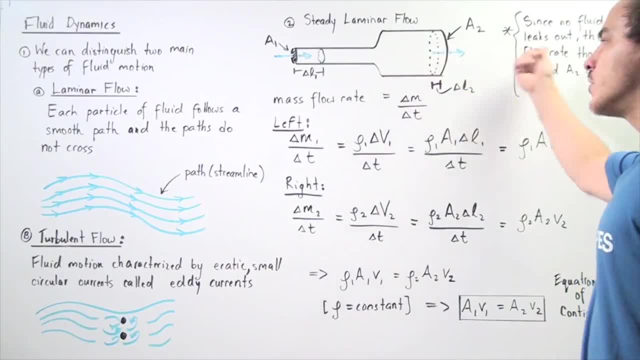 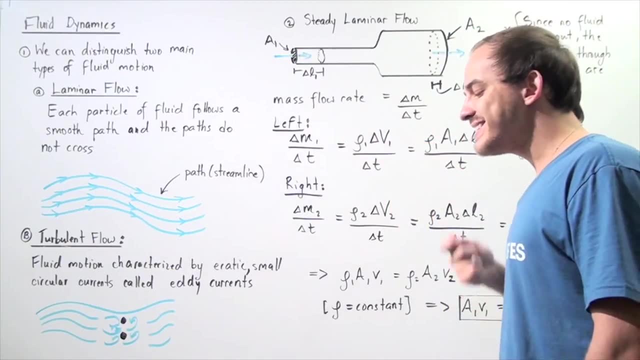 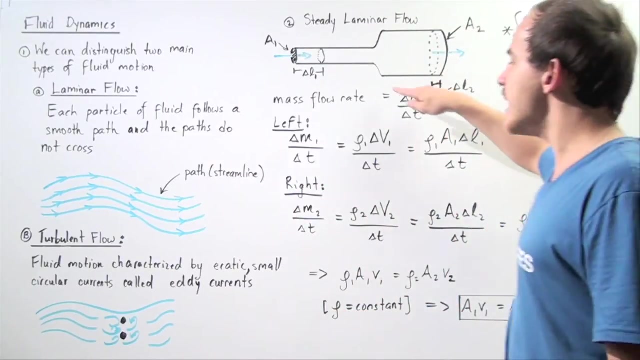 that same amount of fluid comes out from the other end. So let's begin by defining what the mass flow rate is. The mass flow rate is simply the amount of mass of the fluid that passes over some time interval, And the equation for the mass flow rate is simply the amount of mass of the fluid that passes over some time interval. 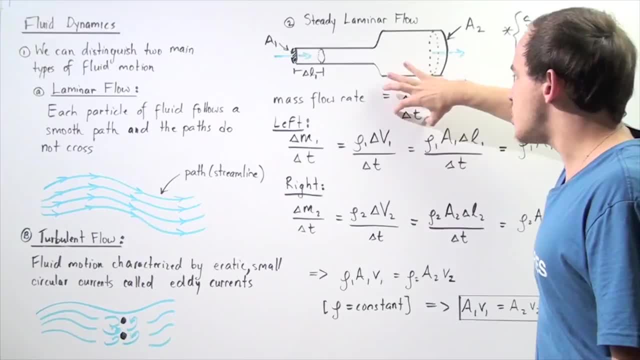 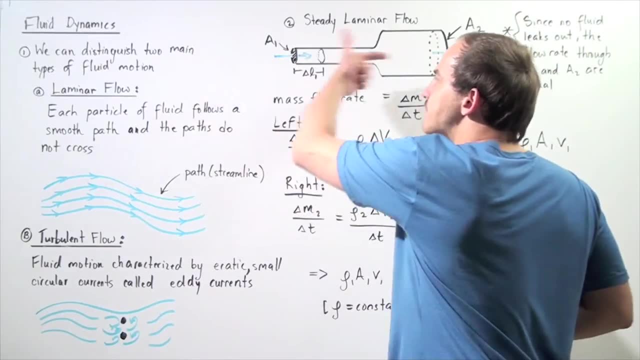 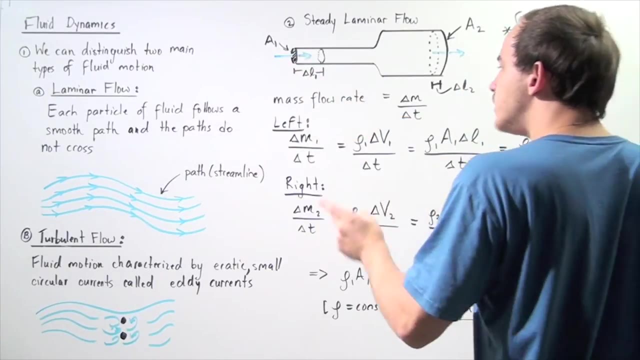 rate is simply change in mass divided by change in time. So let's begin by trying to determine the mass flow rate from the left side of our pipe. So we begin with the left side, this side, and let's label all the terms with one. So one represents the left side, where a1 is the cross. 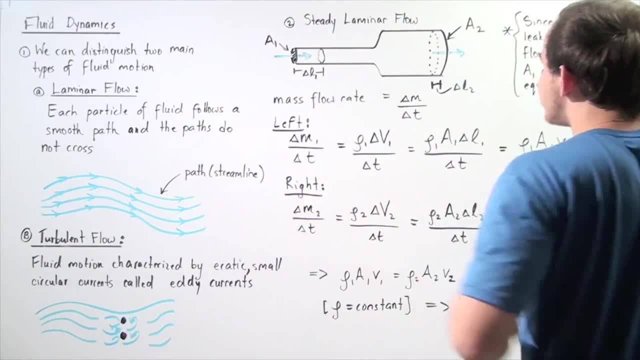 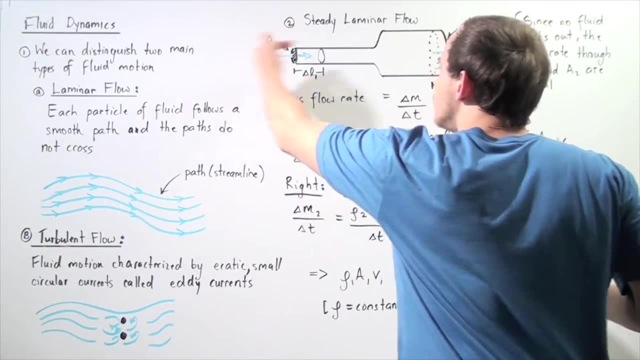 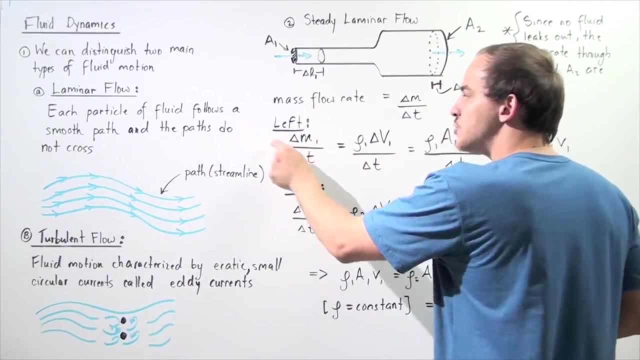 section area of the left side and the right side is represented by the numeral 2.. So let's begin with the mass flow rate through the left side of our pipe. So that means the change in mass of our fluid, change in mass m1 on the left side over the change in time. This is how much. 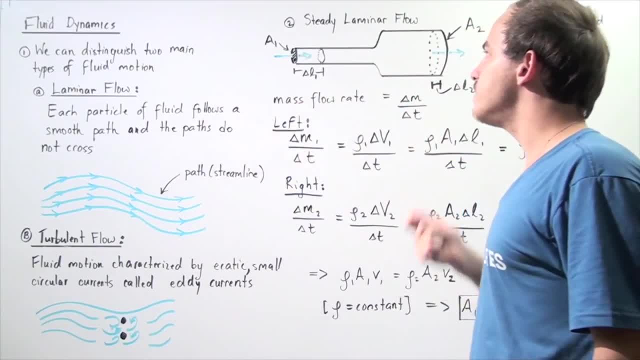 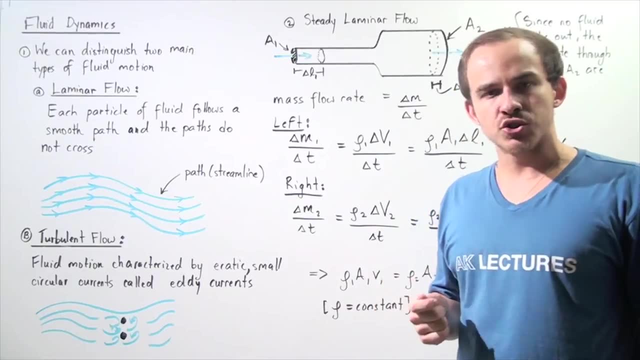 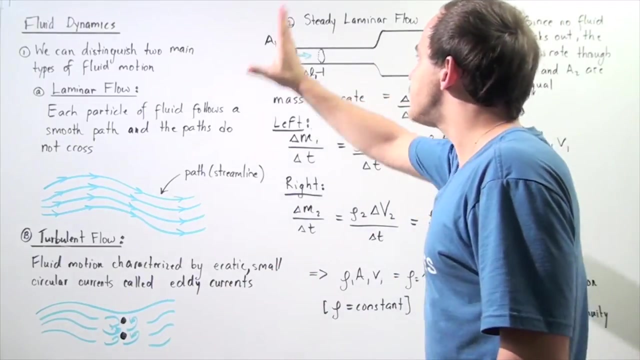 mass of fluid flows on the left side over some given amount of time. Now, what exactly is mass? Well, the mass of the fluid is equal to the density of that fluid multiplied by the volume. So the density on the left side of the pipe, density 1,. 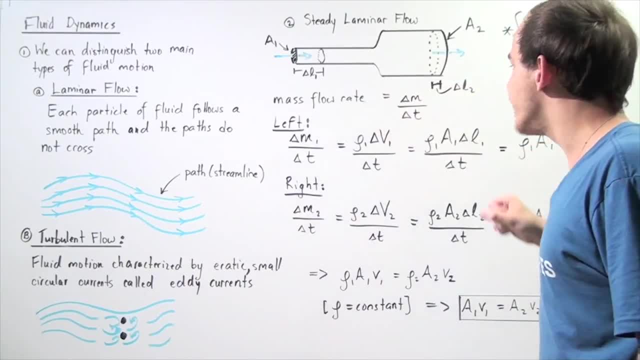 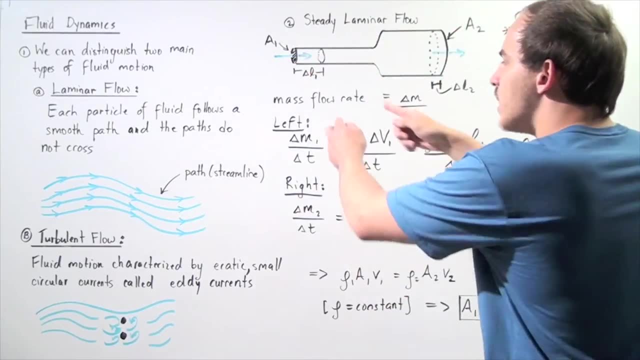 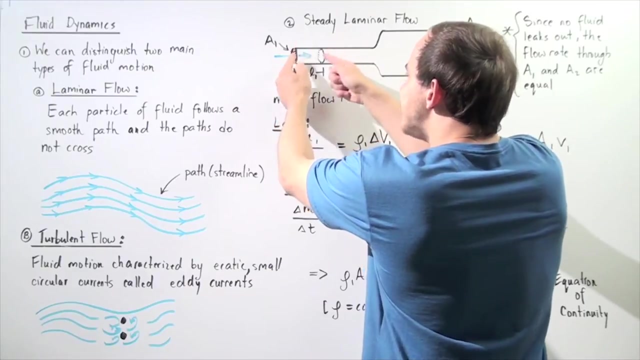 multiplied by the change in volume, v1.. And the change in volume is simply equal to the cross sectional area multiplied by the length that we are considering. So let's suppose we have this much mass of liquid. this much liquid moves this distance over this time. 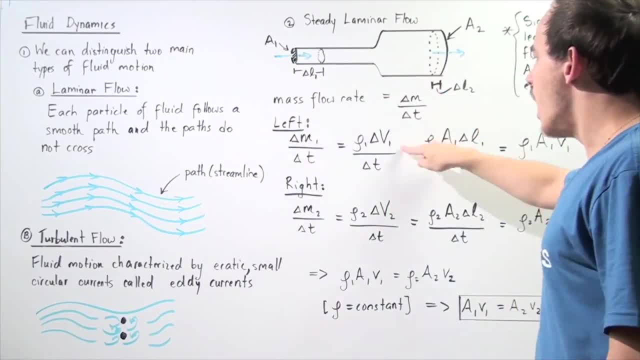 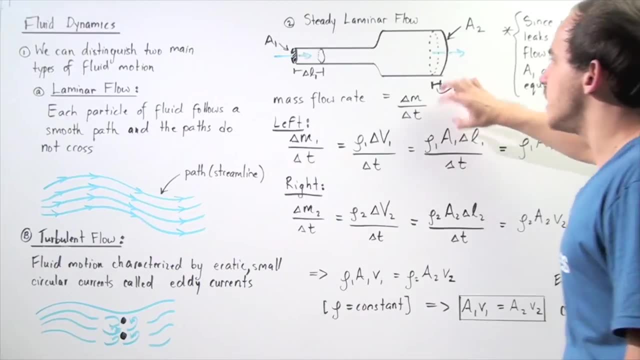 interval. So that means our change in volume 1, on the left side becomes our density 1, multiplied by the cross-sectional area on the left side, multiplied by the distance, our fluid flows change in L1, divided by our time. 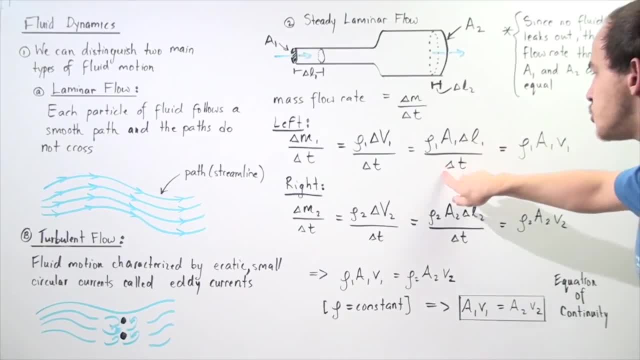 Now notice the change in L divided by change in time is our displacement divided by time, and this is simply our velocity. So we see that the mass flow rate on the left side of our pipe is equal to the density of the fluid on the. 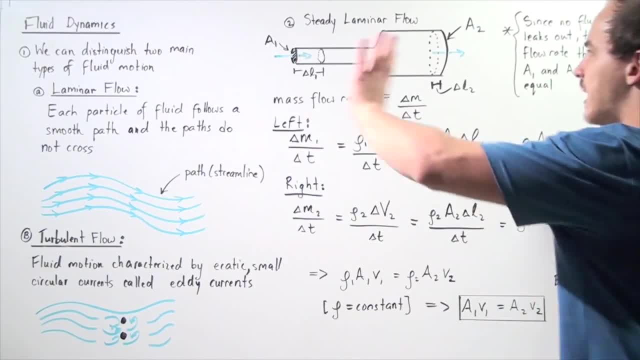 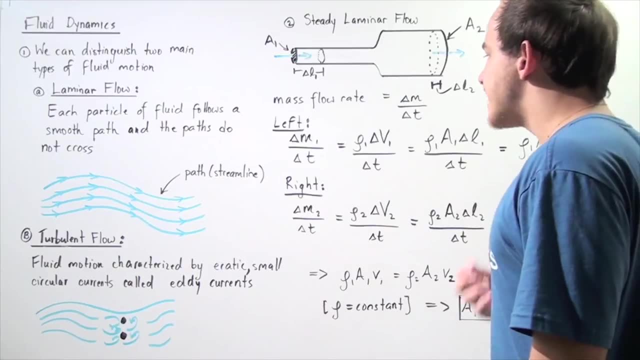 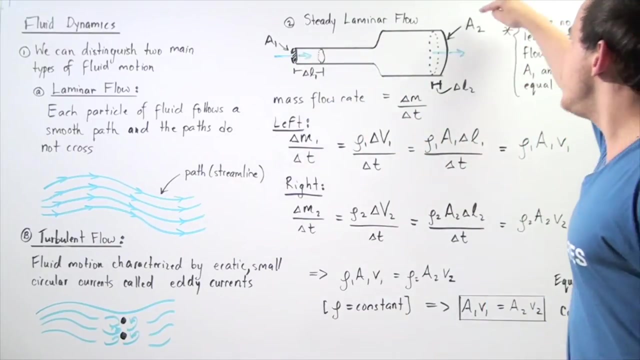 left side, multiplied by the cross-sectional area on the left side, multiplied by the velocity on the left side. Now let's follow the same example. This is the same exact procedure for the right side of our pipe. So this is our fluid leaving our pipe via the cross-sectional area A2.. So we follow the 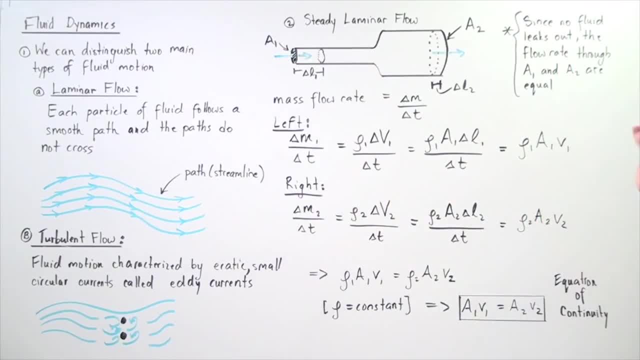 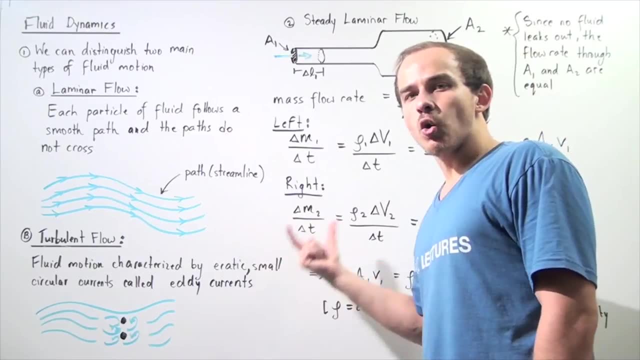 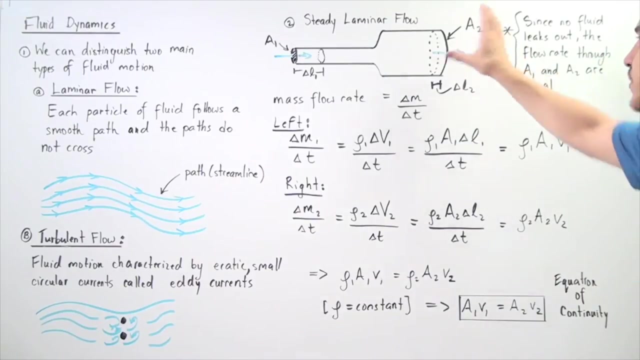 same exact steps and we get the same exact formula, except now we replace our subscripts with 2.. So we see that the mass flow rate of our fluid across the right side of our pipe is equal to the density at that side, times the 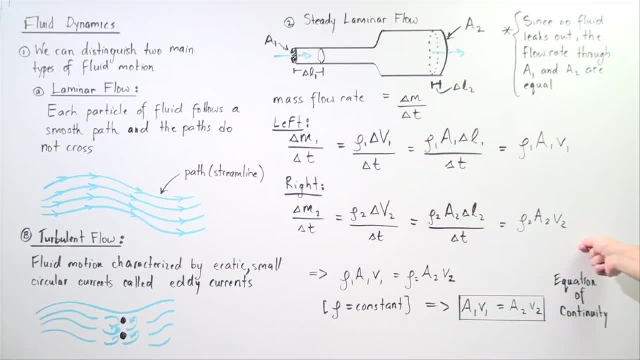 density on the left side multiplied by the cross-sectional area on the left side, the cross-sectional area A2, times the velocity V2.. So we get the following important equation: Why? Well, because the flow rates through A1 and A2 are exactly.